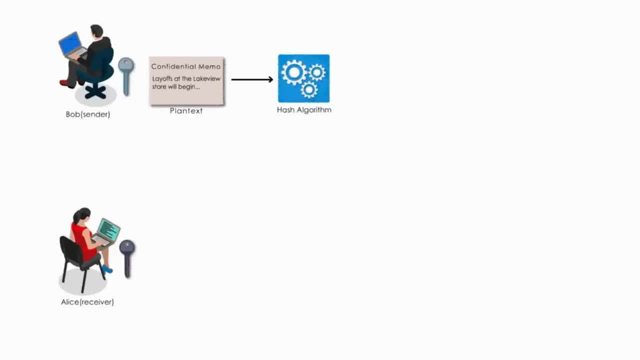 Bob generates a digest by hashing his memo using some hash algorithm. Bob then encrypts the digest with his private key. This encrypted digest is the digital signature for the memo. Bob sends both the memo and digital signature to Alice. Notice: here the memo is not encrypted. 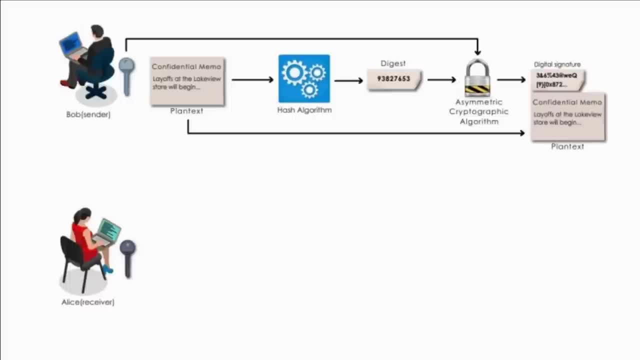 We only focus on the digital signature. When Alice receives them, she will do two things: 1. Alice decrypts the digital signature using Bob's public key and she gets the digest. If she cannot decrypt the digital signature, then she knows it did not come from Bob. 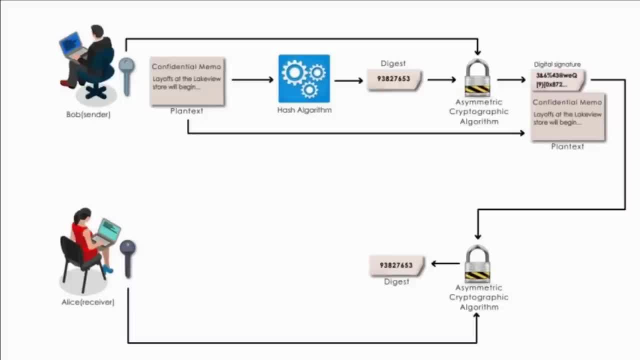 because only Bob's public key is able to decrypt the digest generated with his private key. 2. Once Alice gets the digest, she will check the integrity of the memo. Here is what she does: Alice hashes the memo with the same hash algorithm Bob used. 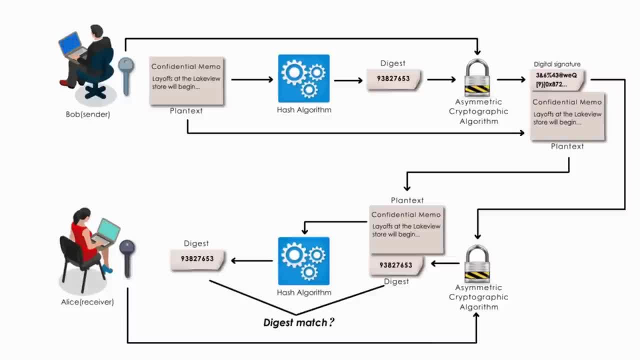 and compares the result to the digest she received. If they are equal, Alice can be confident that the memo has not changed since Bob signed the memo. If the digest are not equal, Alice will know the memo has changed If the digest are not equal. 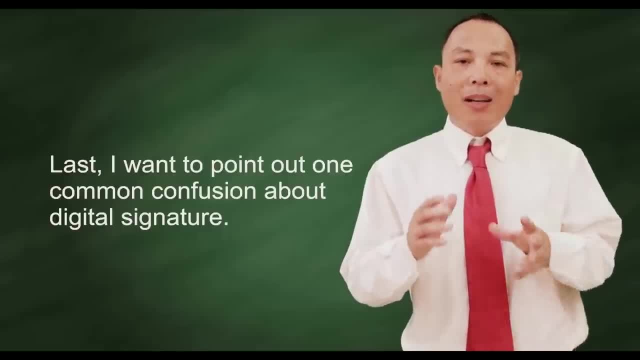 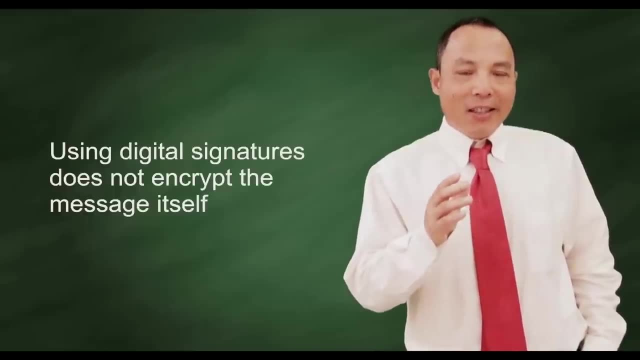 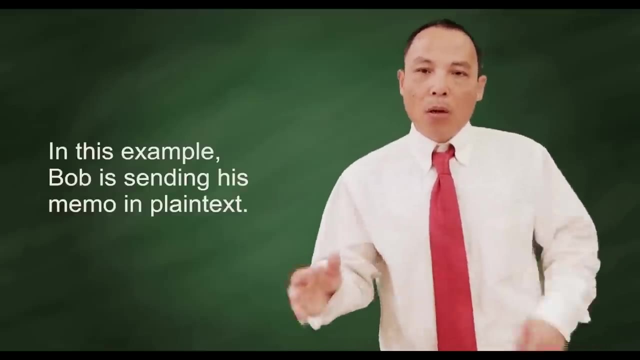 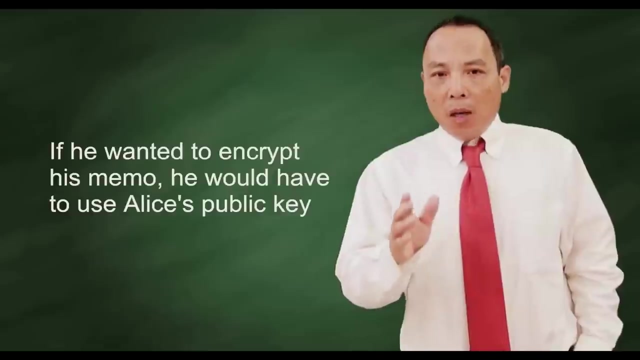 Alice will know the memo has changed in transit. Last, I want to point out one common confusion about digital signature. Using digital signature does not encrypt the message itself. In this example, Bob is sending his plaintext memo to Alice. If he wanted to encrypt his memo. 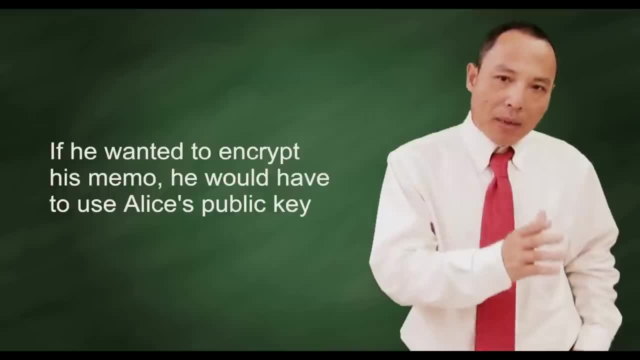 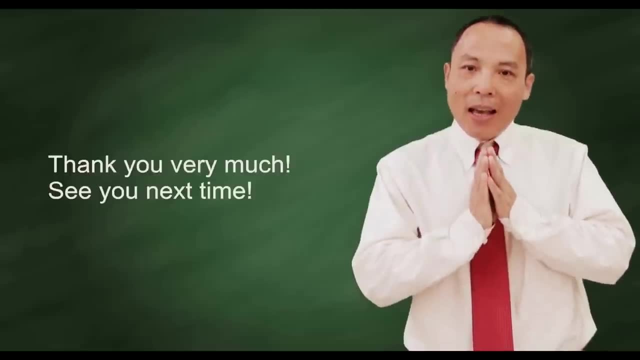 he would have to use Alice's public key, which is another story in another video. Thank you very much and see you next time.